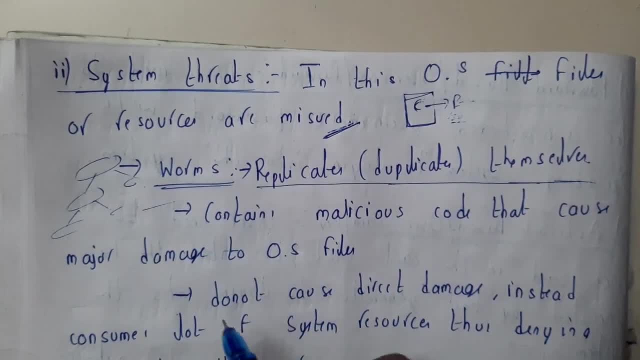 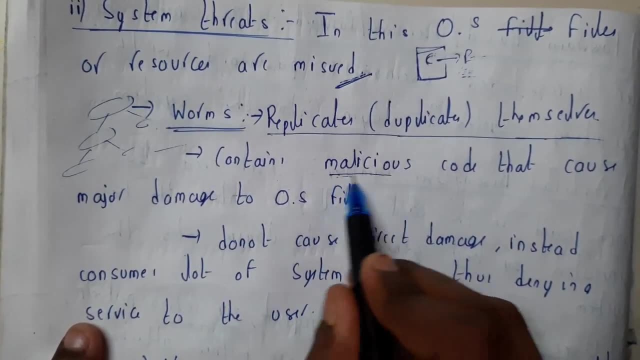 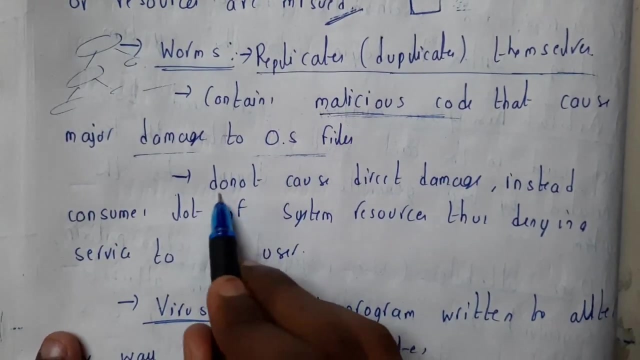 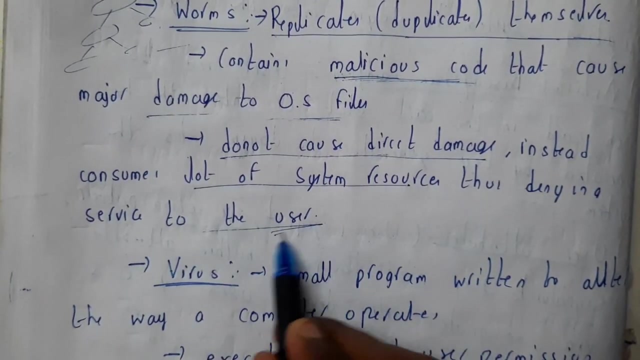 these two worms become these two and these two this. they become four, like eight, sixteen, like that. they duplicate themselves themselves themselves, okay, and they contain a dangerous code that may damage our operating system files, but they do not cause any direct damage. instead, they consume lot of system resources, thus denying the services of 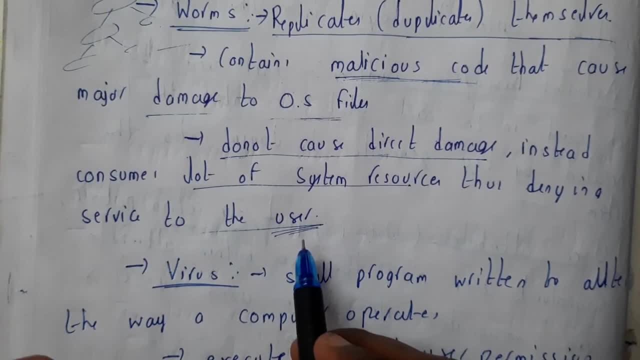 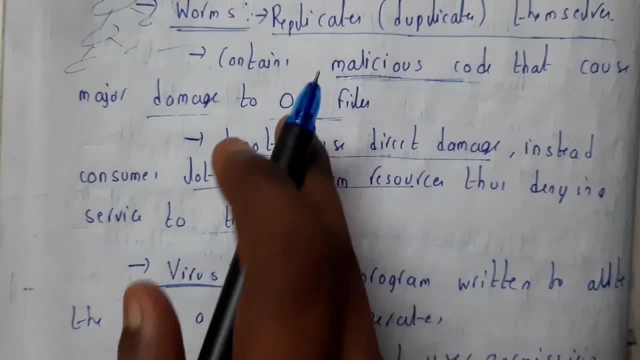 user, so they are not able to run the system. they are not able to run the system. they are not able to run the system, so your system, usually it will spruck right when you are opening multiple files or multiple browser tabs or anything. it may struck for a minute second so that is because of this worms. basically, these are the things. 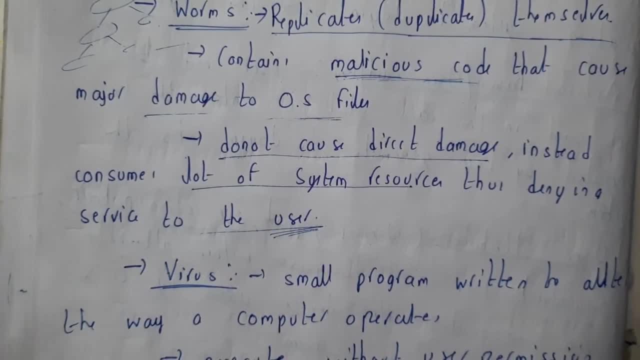 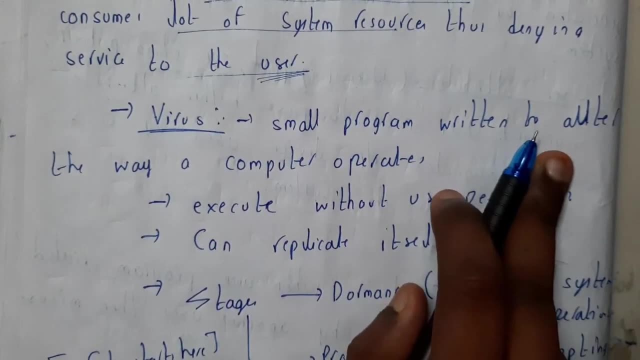 which, whatever you antivirus you may use, these worms will exist, guys. basically, so virus, so virus. virus are the small programs, return by return to alter the way a computer operates. so these viruses can alter the way a computer operates. so these viruses can get the support of a computer. the computer can get the support of a computer. 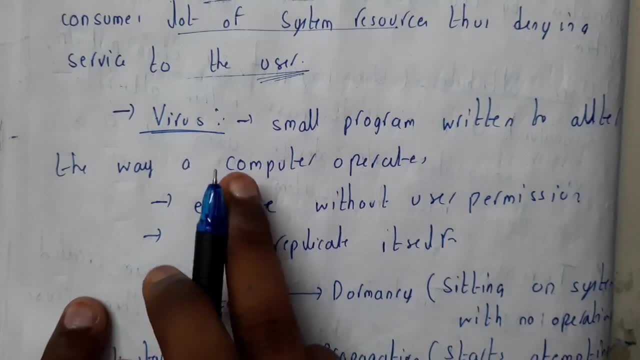 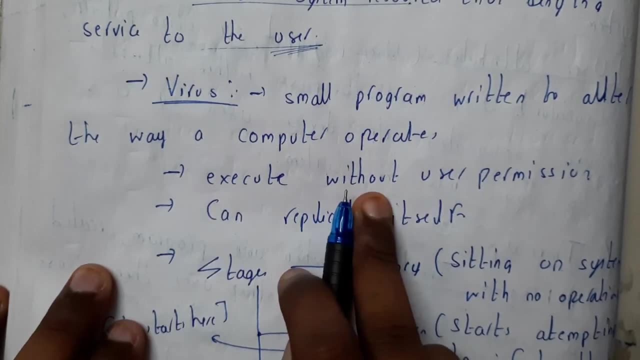 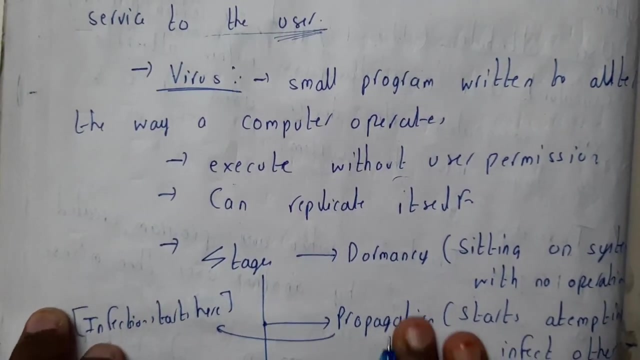 二, three, four, five, six, seven, twenty, twenty, seventy, seventy, thirty change the way how your computer is operating, so they can change the execution permissions and they can execute without the user permission. they can open files, they can transfer data, they can copy files, they can do anything they want, and these viruses can also be replicating themselves. 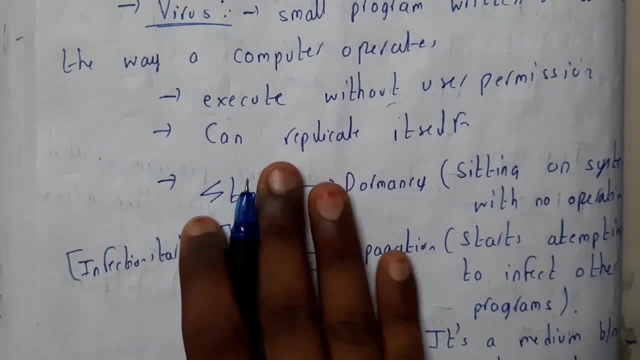 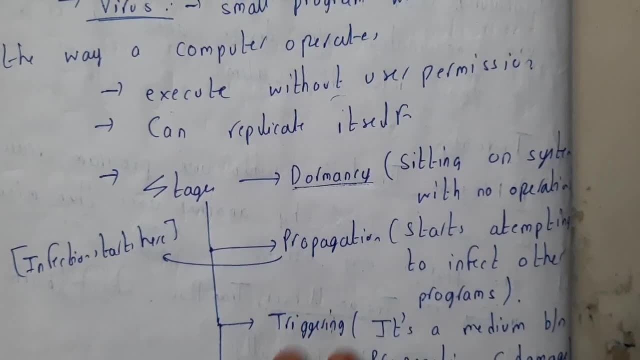 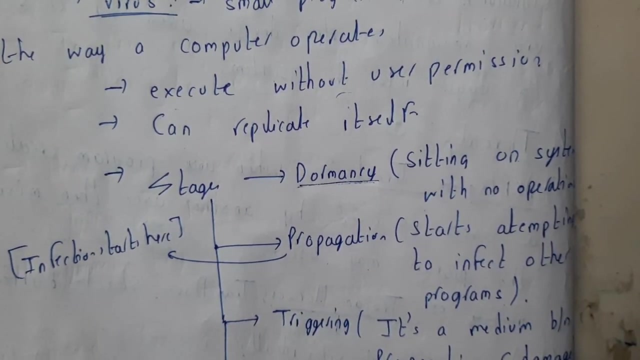 fine, so there are four stages for viruses, guys. so basically they will be in dormancy stage. dormancy is nothing, but dormancy stage is nothing. but the virus initially will be staying in the system and it will monitor everything else. it will not react or it will not do any operation. 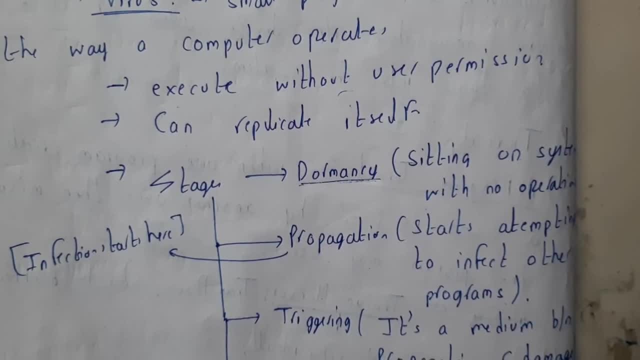 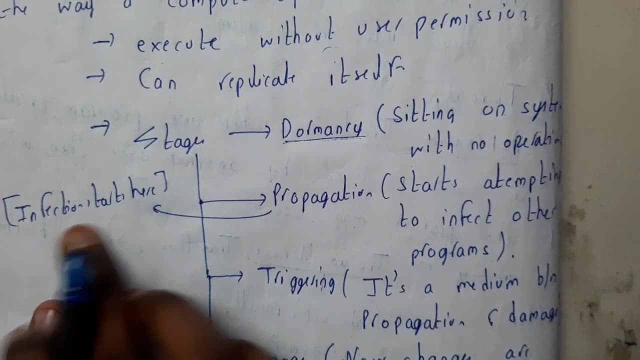 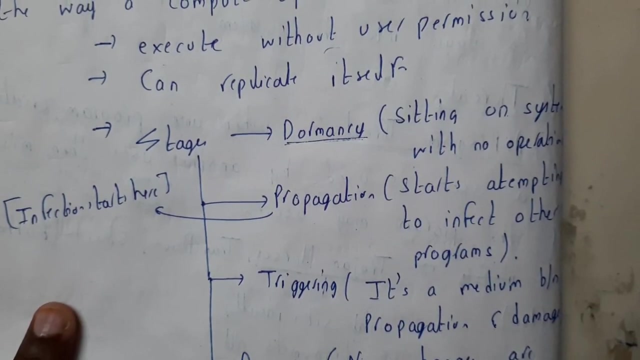 it will be just sitting in a system at a some random place and it will be monitoring everything. and the second stage will be propagation. propagation is the place where the infection starts. it starts trying to trying to. it will try to attach or it will try to attack some programs. 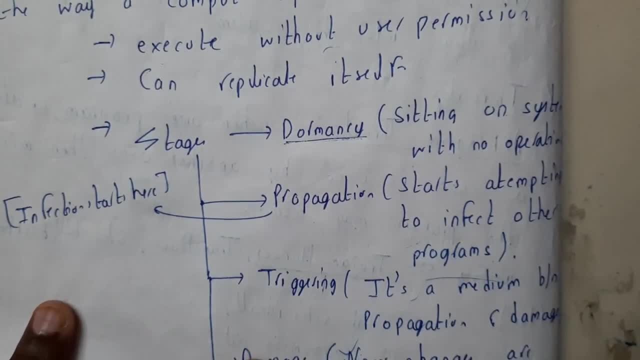 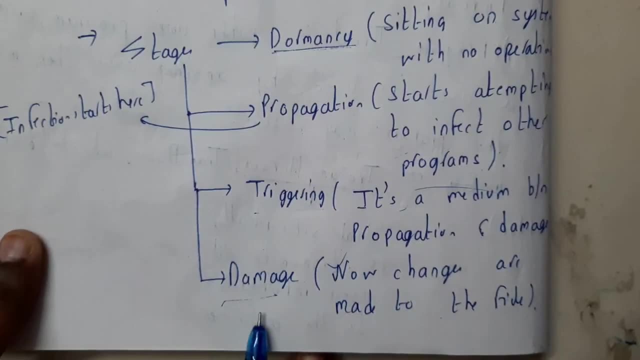 so starts attempting to inter interact with other programs or interface with other programs. so then comes the trigger. trigger is nothing but the medium between the propagation and damage. fine, so damage. damage is nothing but at the place, where at which the file is damaged. now, so this is the final stage at which it will.